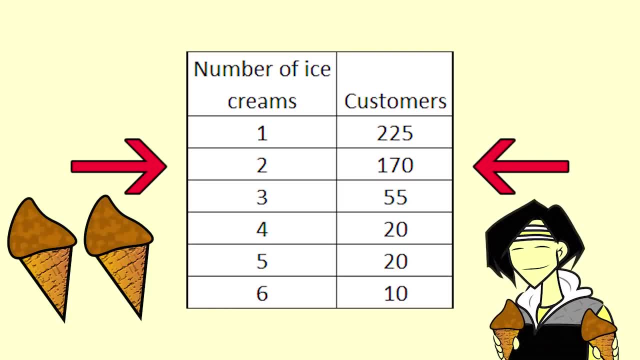 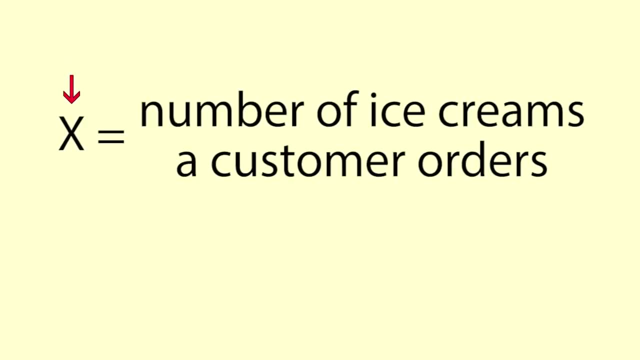 of ice creams bought and the number of customers who bought that number of ice creams. We can define X as being the number of ice creams a customer orders. X is a random variable. It is called random because it can take several different values and is the result of a chance happening. We estimate the 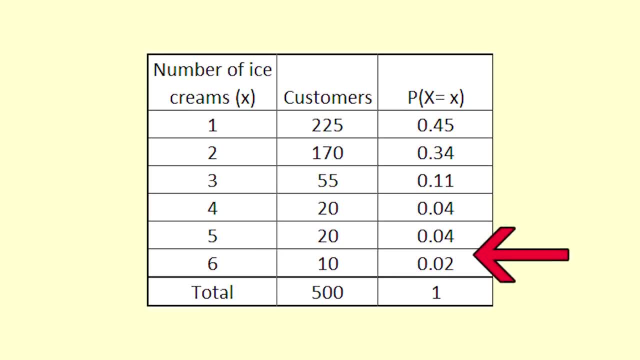 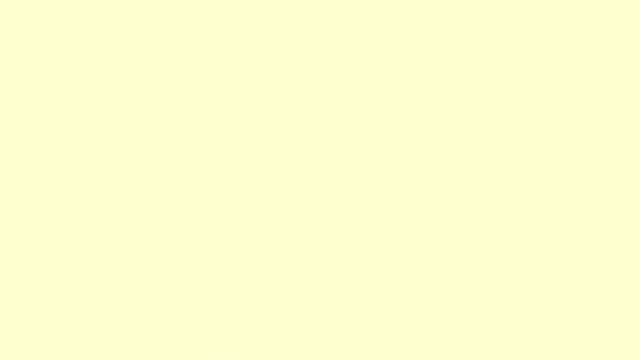 probability for each value of X by finding the relative frequencies for the number of ice creams one customer buys from the historic or experimental data. The distribution for X- the number of ice creams one customer buys- looks like this As a dot diagram, it looks like this, which could be rearranged to: 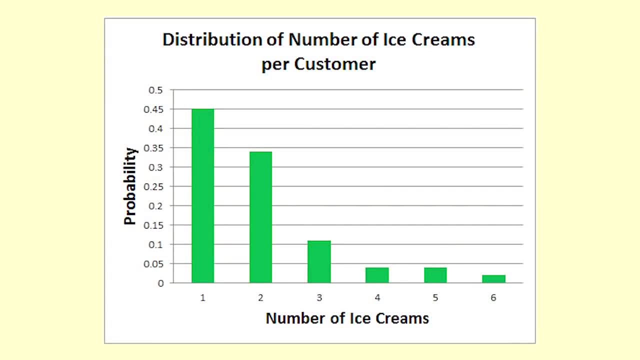 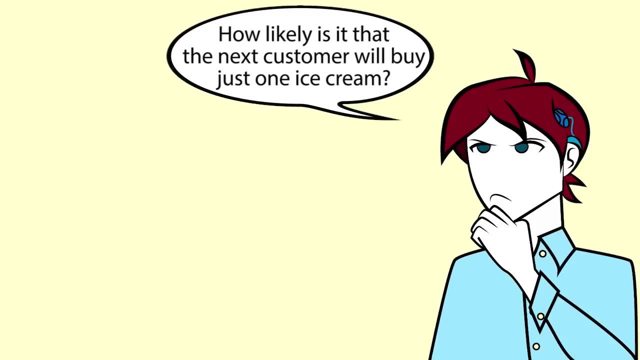 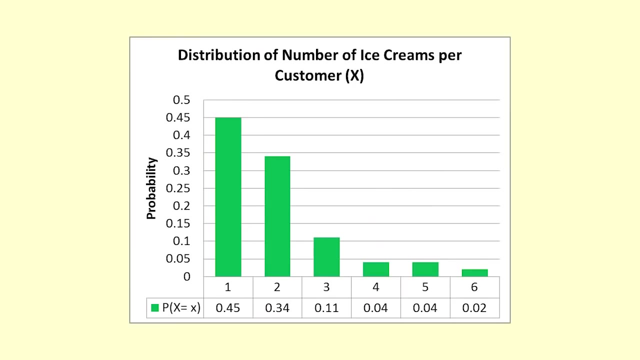 look like this. We often like to show distributions as a graph. We can use this distribution to answer questions. Luke wants to know what is the probability that the next customer will buy exactly one ice cream. We look on the table and tell him that the probability that X equals one equals .45 or forty-five percent. 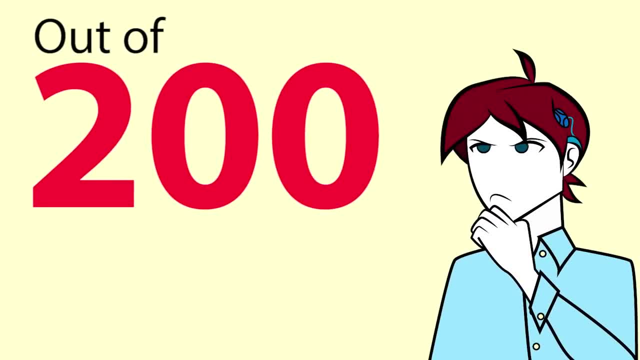 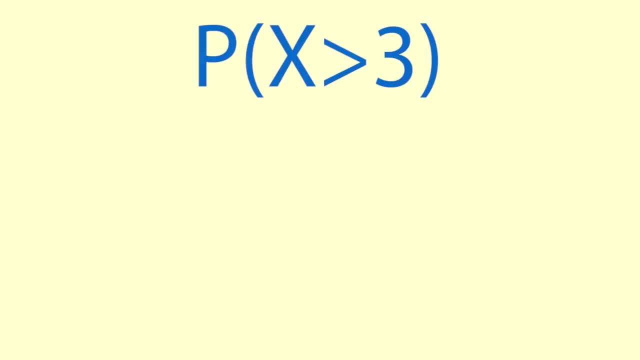 Luke then asks: out of two hundred customers, how many would we expect to buy more than three ice creams? We want to find the probability that X is greater than three, so we add up all the probabilities that apply The probability that X is. 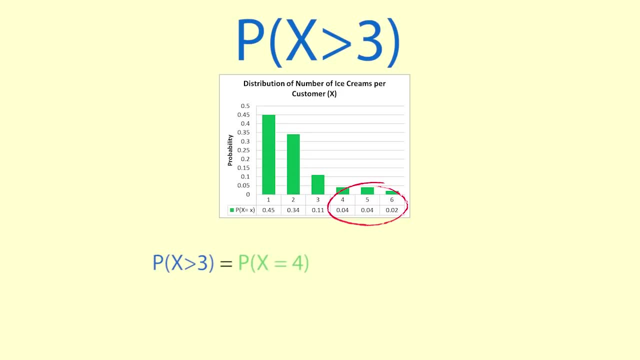 greater than 3, equals the probability that x equals 4 plus the probability that x equals 5 plus the probability that x equals 6, which equals 0.04 plus 0.04 plus 0.02, which equals 0.1 or 10%. 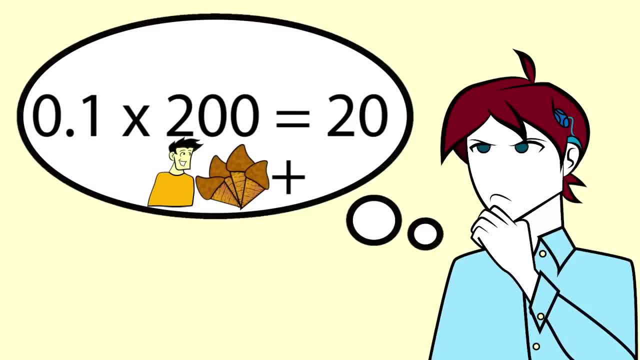 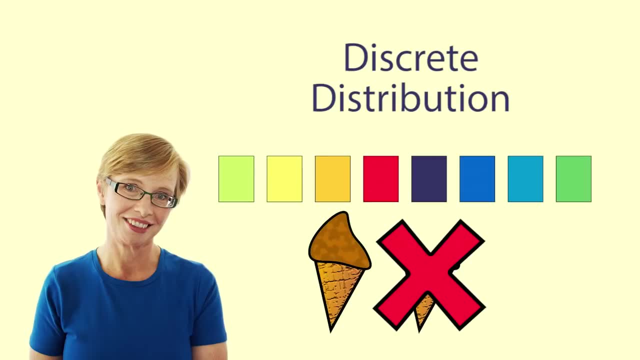 0.1 times 200 equals 20, so we would expect 20 customers out of the next 200 to buy more than three ice creams. This example of number of ice creams is an example of a discrete distribution, as you can only get whole numbers of ice creams. Other things that can be modelled as discrete. 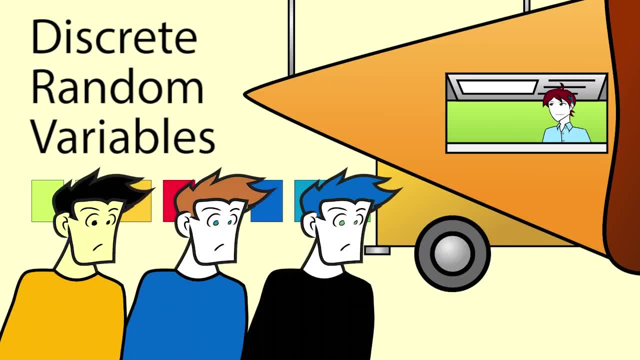 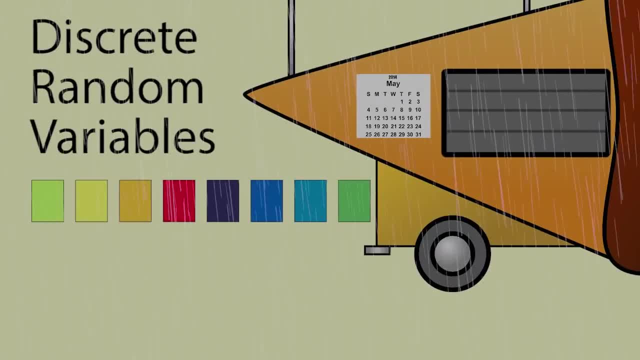 random variables are: number of customers who arrive in the next hour. number of customers who pay by cash. number of days in a month in which the stall is closed due to rain. number of cones that break while being filled. The following cannot be used to define the number of customers who arrive in the next hour.